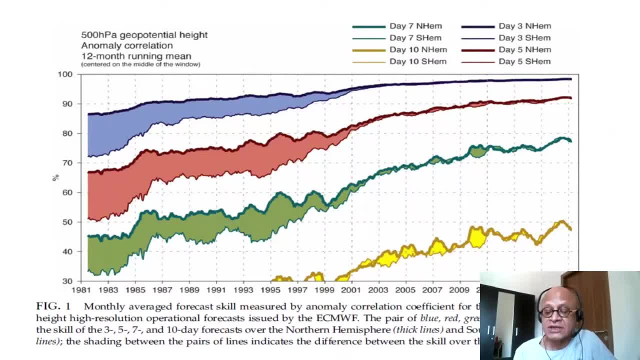 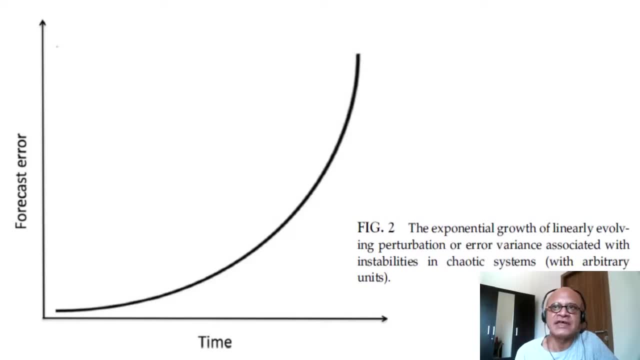 So Southern Hemisphere, which has more ocean, suffered from that as well. In general, when you have a system which has some Stability in it, it can have a chaotic behavior which, in terms of forecasting, you can think of it as exponential growth of linearly evolving perturbation or error variance associated with instabilities in a chaotic system. 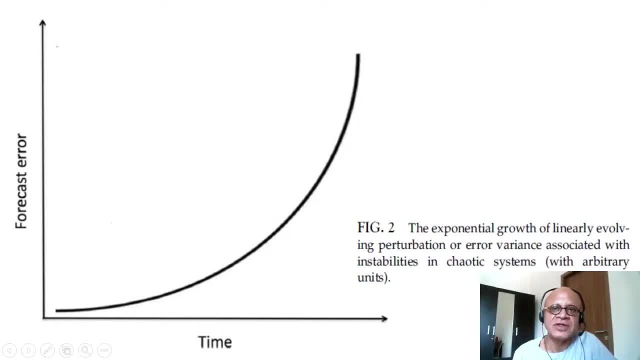 So you can just write some exponential relation for a particular variable with the growth factor And it tells you how small perturbations or Chaotic behavior of the system itself can give you growth in error, which basically kills the prediction skill after some time. 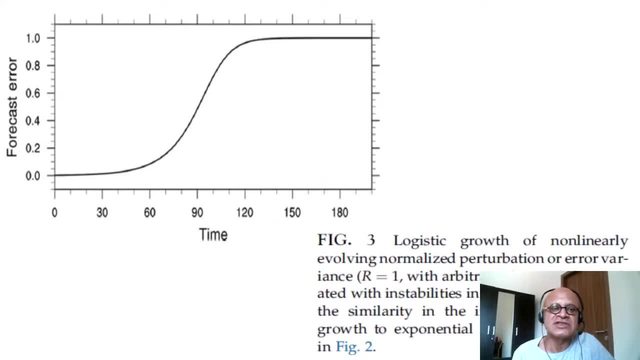 But it turns out that if you have a nonlinear system you can saturate the error over a longer time. So you can see that there is a similar growth in forecast error, but then it gets saturated somewhere up here, which on long time scale, basically all predictability is lost. 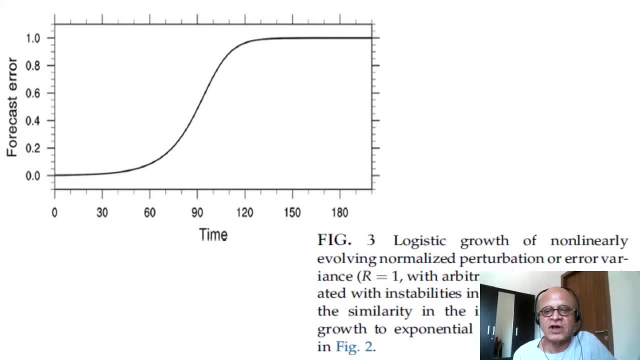 A good example would be to think of, let's say, a seasonally dependent error growth which can get saturated when the season changes, because there are nonlinear interactions between background state change because of seasons and the process- weather process- that you are looking at. 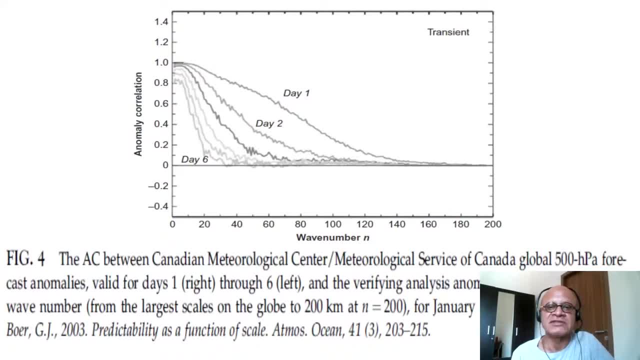 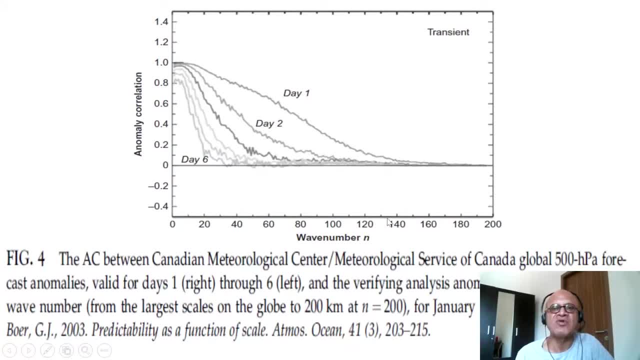 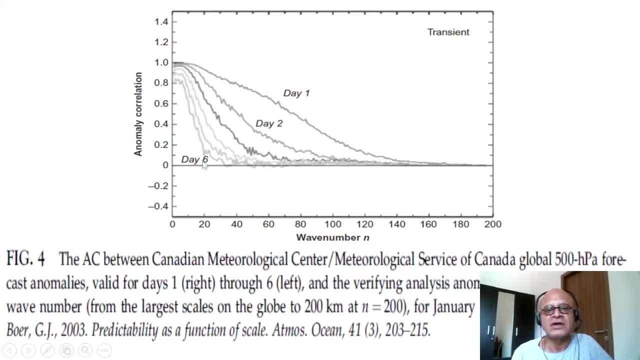 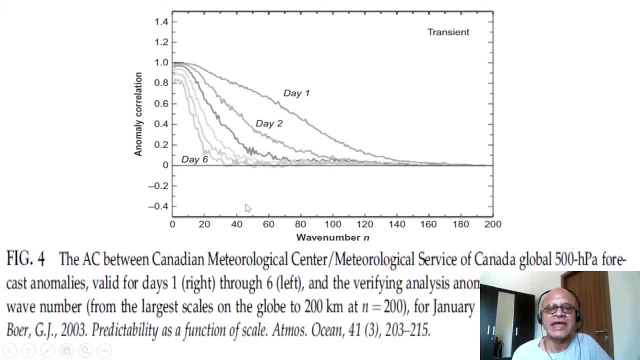 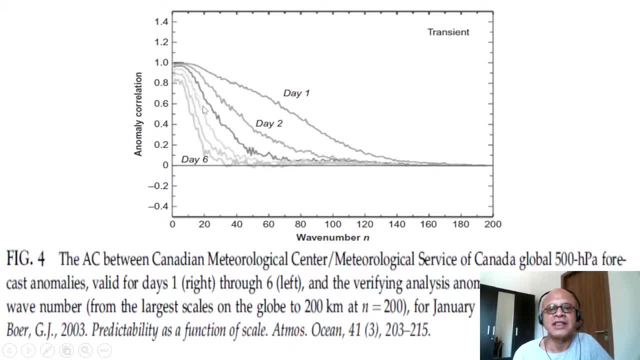 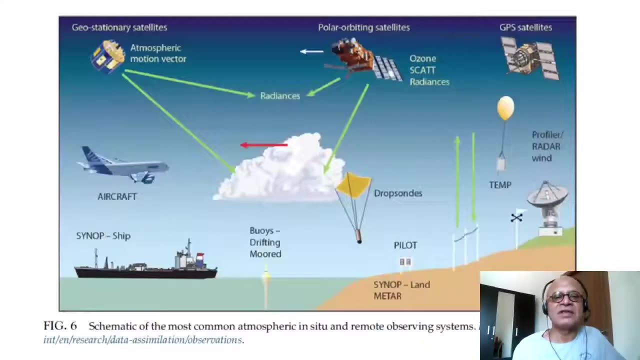 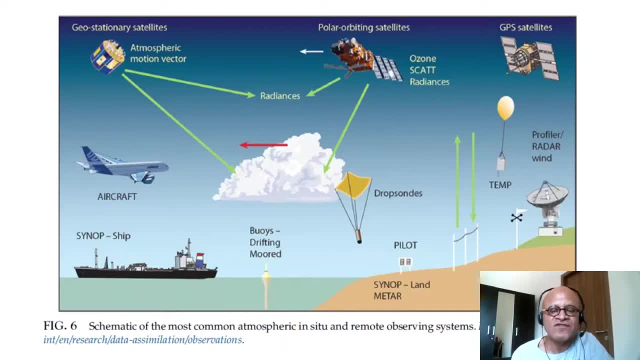